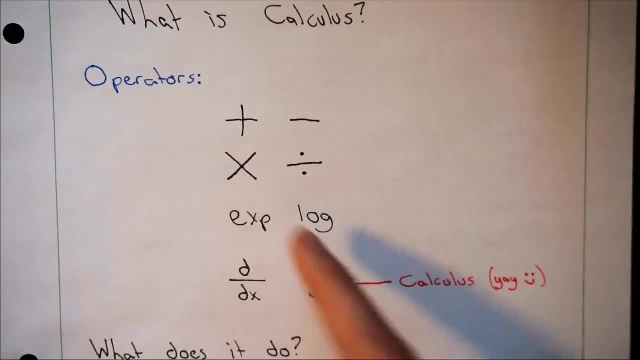 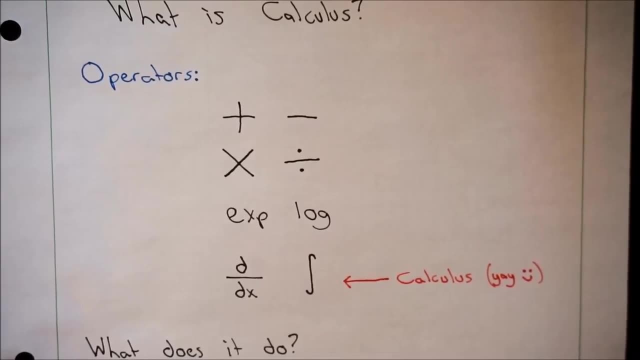 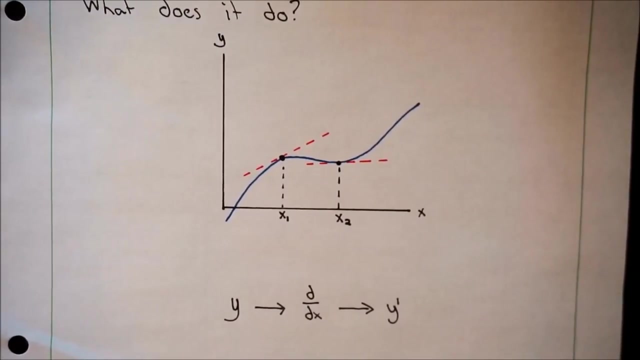 So minus is the opposite of plus, Division is the opposite of multiplication. Well, integrals are the opposite of derivatives. They're sometimes even called antiderivatives. And what do they do Sometimes in physics, you'll have a graph of something like this. Let's say: 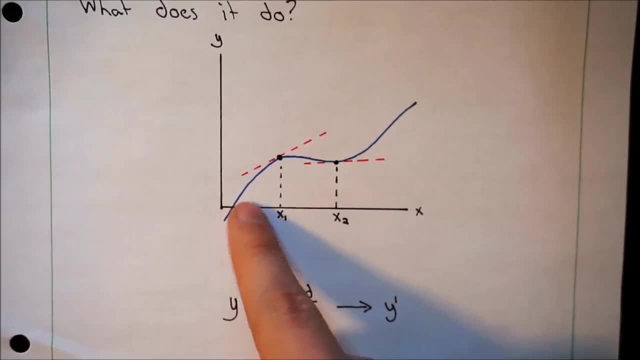 this is position. So we've tracked the position of an object and we've graphed it here. In this case, this would be time and this would be distance. Now, if you wanted to find the speed of the object at any one time, 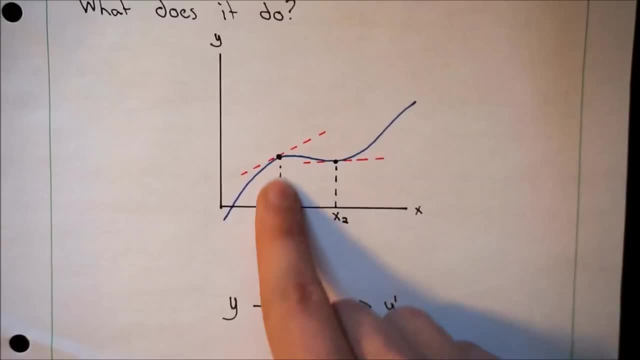 you would have to find the slope of the tangent line at that point. Now, the old way of doing it would be to draw a tangent line on it, like I have here, and then you would just measure the slope of this line to figure out how fast it's going. 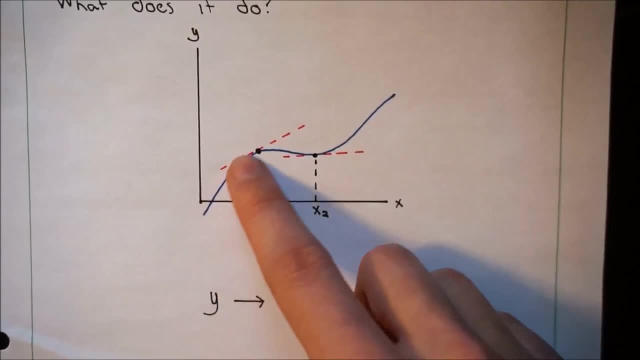 With calculus you can take the equation for this blue line which we call y here. If you take the derivative of that, it'll spit out another equation we call y prime. And what you can do with y prime is take any point on this line. 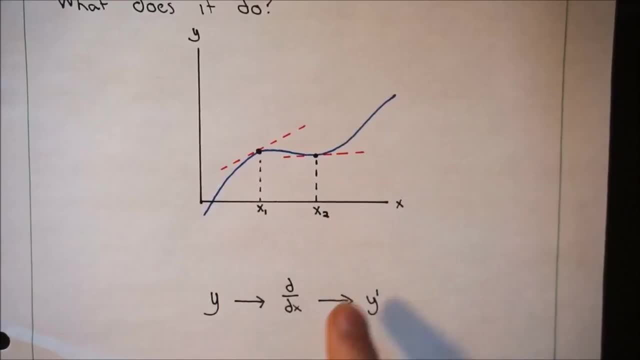 Let's say we want x1.. Let's say x1 is 2.. You would take 2, put it into your y prime equation and it would give you the slope of this tangent line at that point. So you can do that for x2, you could do that for. 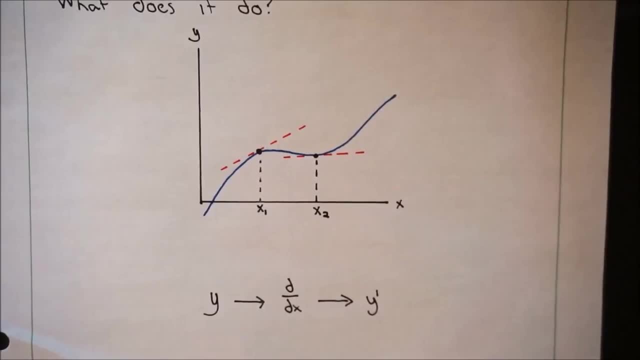 any point along this line. It's very, very handy and it's a lot easier than drawing out tangent lines and trying to measure it. that way It's also a lot more accurate. It gives you a perfectly exact line. So that's the algebraic answer. 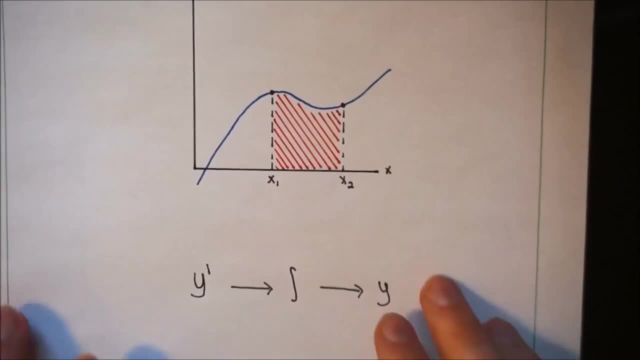 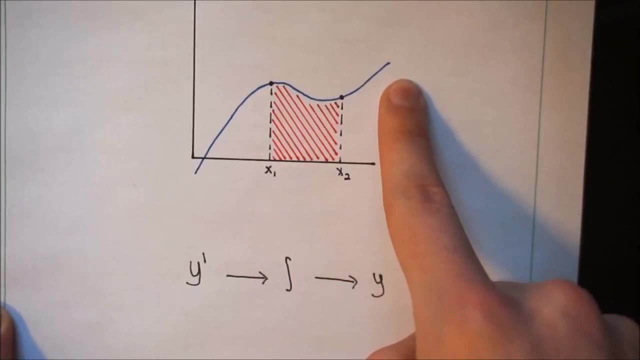 The integral or antiderivative. so in this case our blue line here is the y prime. So let's say this is the velocity, and we want to know how far our object went. So you would have to find the area under the graph and that would give you. 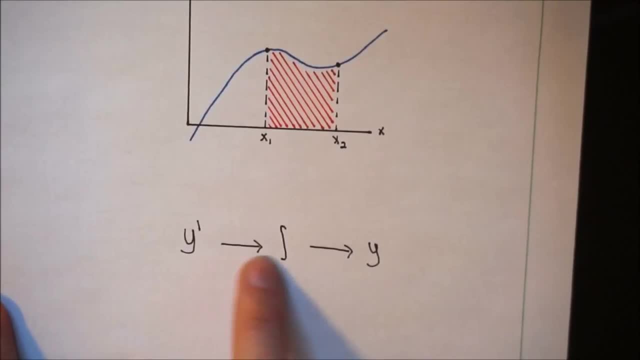 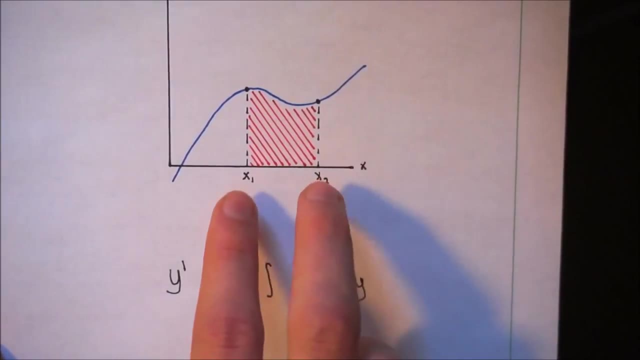 displacement. So you take your integral and it will spit out a new equation for y, And what we do with the integral is typically we'll integrate it with the integral, So you'd actually have to put both of these numbers into the equation here.